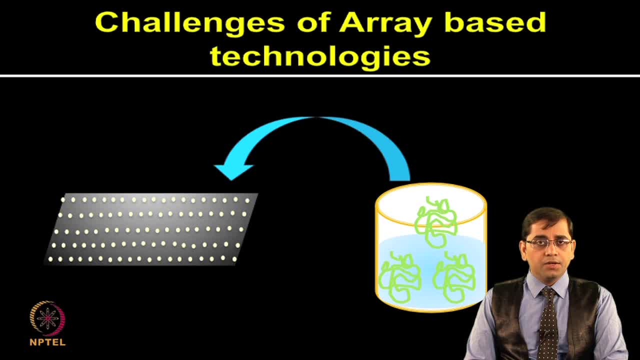 it provides an important platform for large scale functional analysis of proteins. Although, due to the high throughput capabilities, array based proteomics attracted tremendous attention in clinical research, It has quite a few technological challenges as well. Protein array designing difficulties includes acquisition, arraying and stable attachment of proteins to array surfaces. 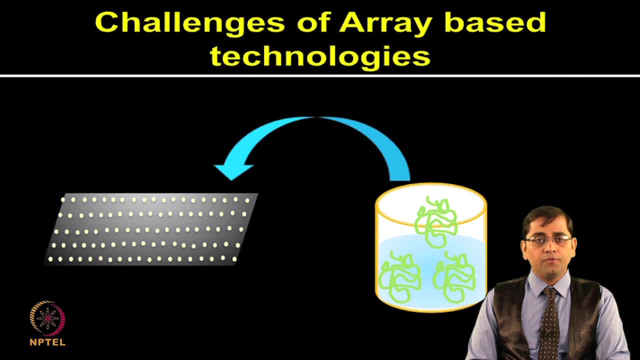 and detection of interacting proteins, Further miniaturization of assays, protein dehydration, non-specific binding, unavailability of highly specific antibodies against all the protein proteins that comprise the complex proteome, and lack of direct correlation between protein abundance and its activity. The complex nature of proteins has posed many hurdles in the 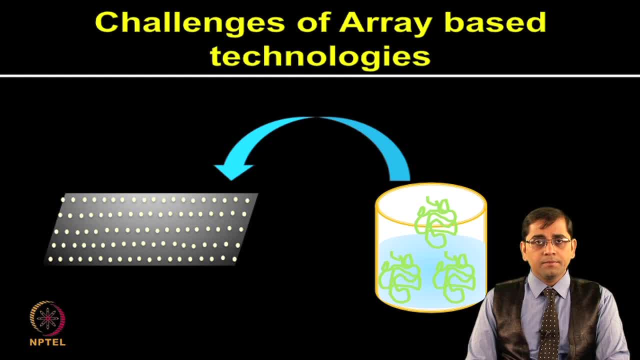 area of array fabrication, printing, scanning and data analysis. DNA microarrays had laid the foundation in developing experimental and analysis strategies. However, DNA microarrays are not the only source of protein abundance. They are also a source of protein toxicity. However, there is an enormous scope for innovation and making protein microarrays more robust. 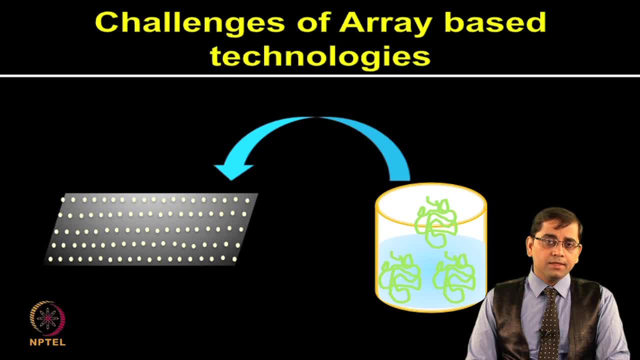 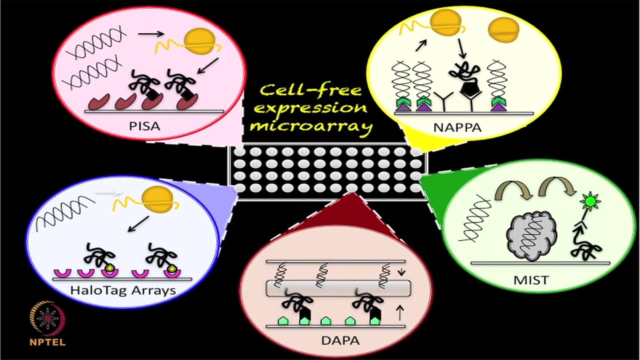 and user friendly. Diversity in protein size, spatial location of proteins in cell post, translation modifications and hydrophobic nature of the proteins pose challenges for protein purification, maintenance of activity and orientation for functional assays using protein microarrays. Technologies like cell-free expression system have helped to overcome the challenges of 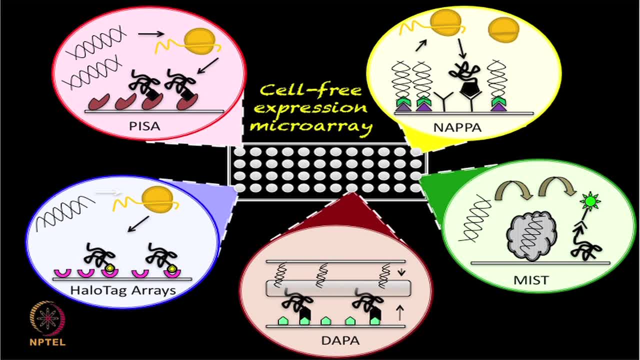 high throughput expression and purification for a diverse class of proteins. Cell-free expression aids in generation of near native configuration of proteins. Nucleic acid, programmable protein arrays and halotrach technologies allow the presentation of hidden or buried epitopes in a protein for development of better assays. Many commercial biochips are. 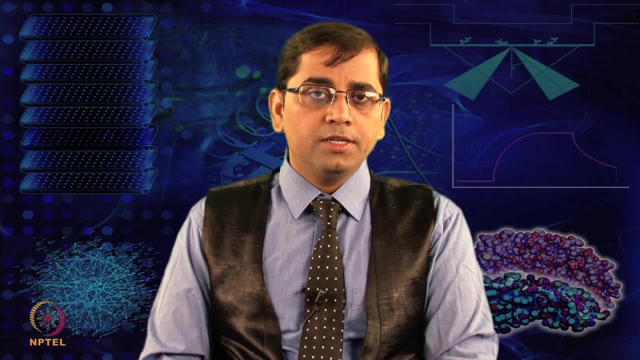 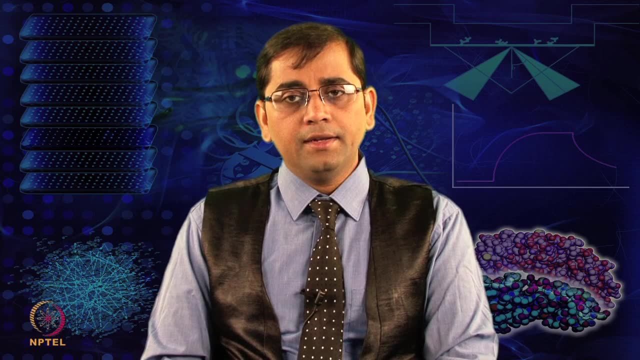 now available for the study of post-translationally modified proteins. Thus, protein microarrays have overcome many of the inherent challenges through innovation in last few years. However, data analysis continues to be an area which could be worked on further in the future. Data analysis continues to be an area which could be worked on further in the future. Data analysis continues to be an area which could be worked on further in the future. Alright, friends, thank you if you have interested in learning about this particular proxy trajectories. 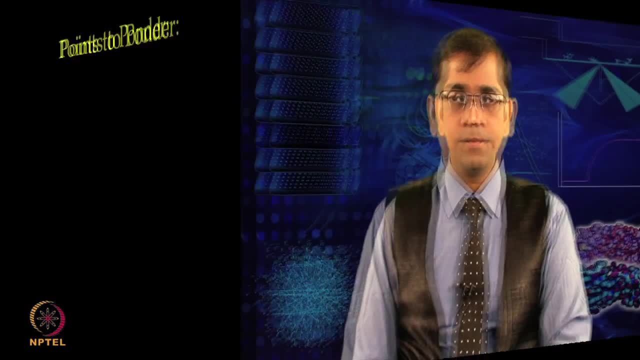 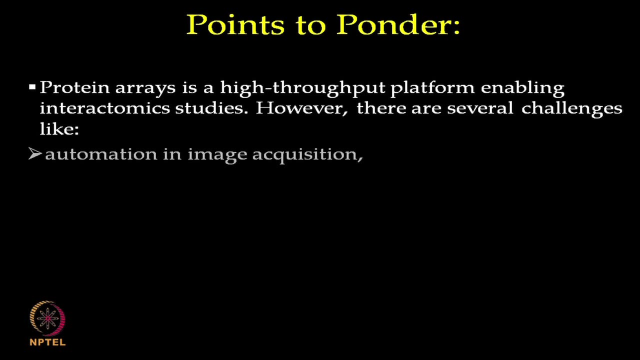 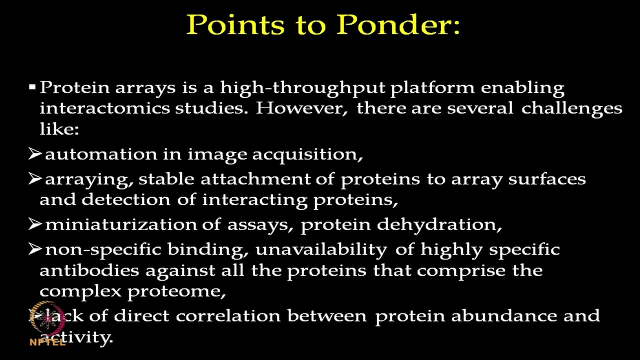 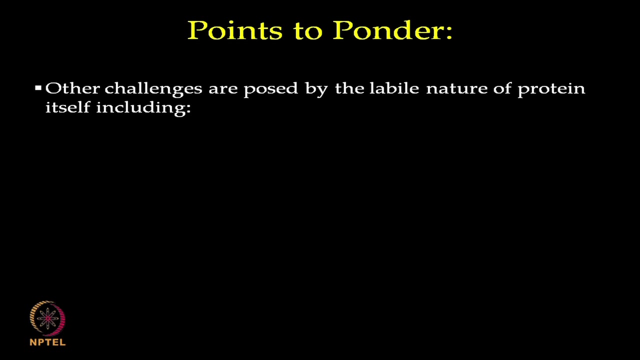 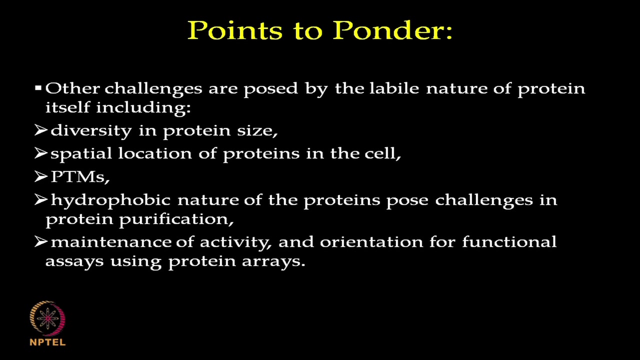 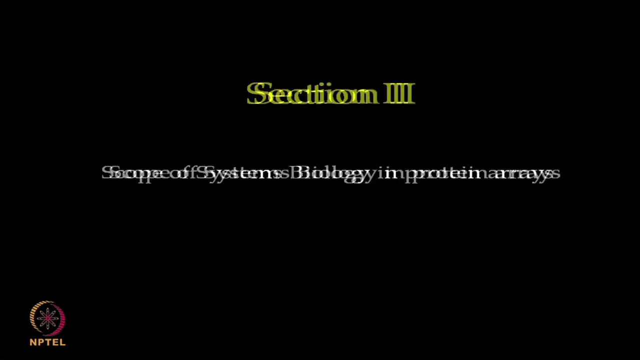 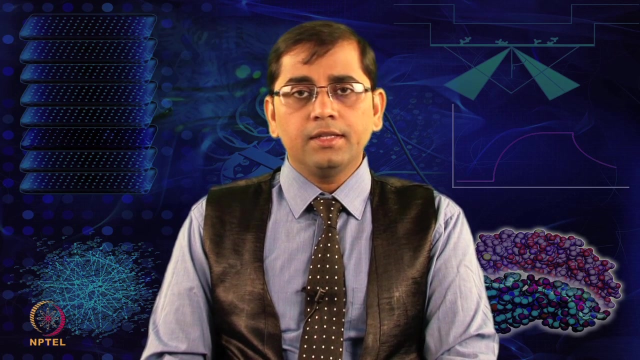 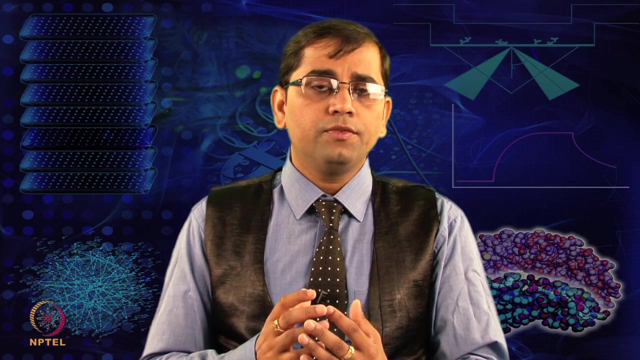 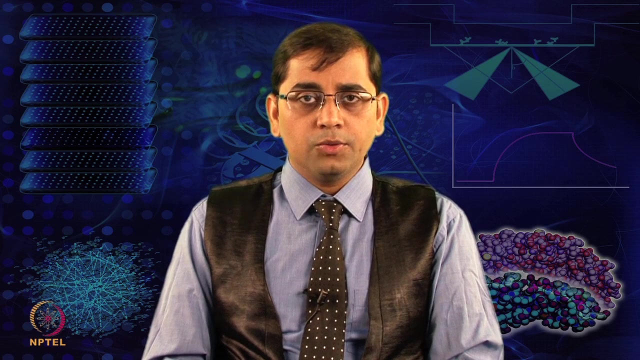 nobody is a genius, Thank you. There are several challenges associated with these high throughput technologies. However, the data from such platforms are indispensable resource for integrative understanding of living systems. This brings us to the last segment of this module, which is known as system. 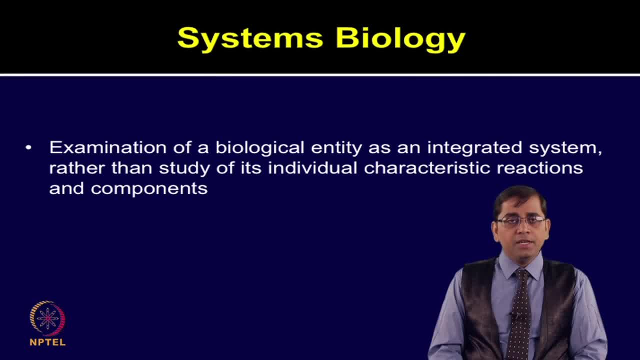 biology. System biology is the examination of a biological entity as an integrated system, rather than a study of its individual characteristic reactions and components, which is termed as system biology. It is a study of all the mechanisms underlying complex biological processes in the form of its interacting components. System level understanding require. 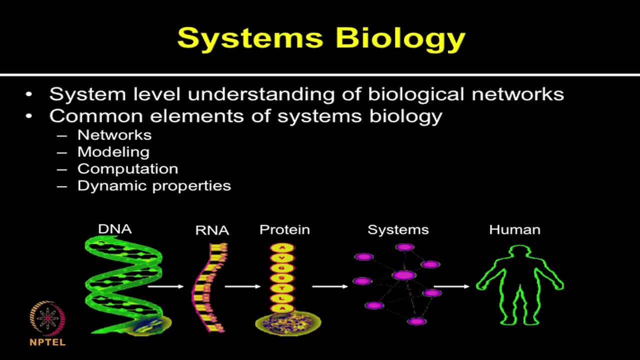 information from different levels at the genome, transcriptome or proteome level, which can then be applied To understand a complex system and also be applied to different organisms. The biological information is represented by the network of interacting elements and dynamic response to the perturbations. These networks provide insights which cannot be analyzed from the 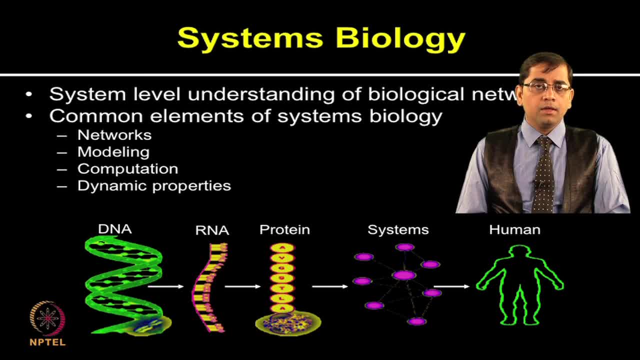 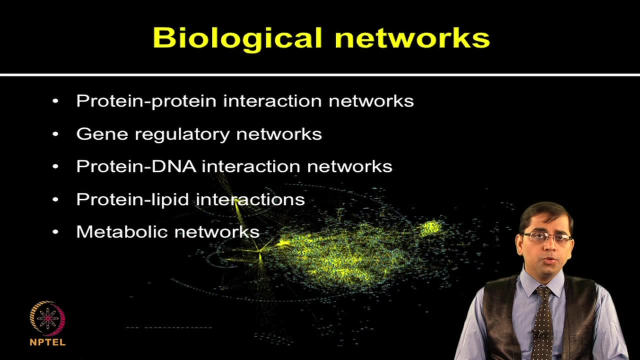 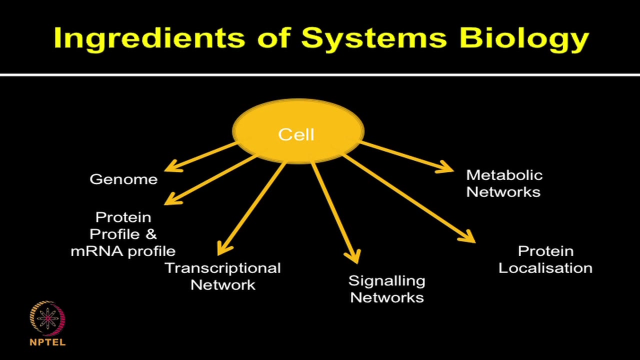 isolated components of the system. The common elements of system biology include networks, modeling, computation and dynamic properties, The different types of biological networks, such as protein-protein interaction networks, gene regulatory networks, protein-DNA interaction networks, protein lipid protein, other biomolecule networks and metabolic networks. If you are studying a cell and its 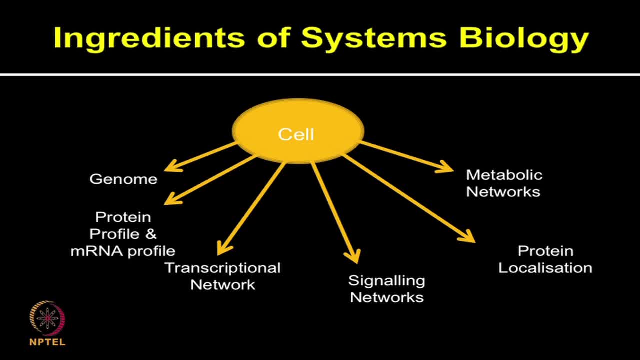 systemic behavior. you need to look at the genome, its transcriptome profile, proteome profile, how protein, DNA and different transcriptional networks are altered, protein-protein signaling networks, multimeric complexes, etc. We need to know how they are formed, how protein is. 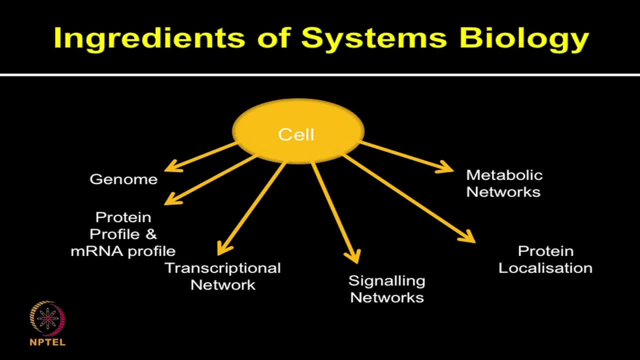 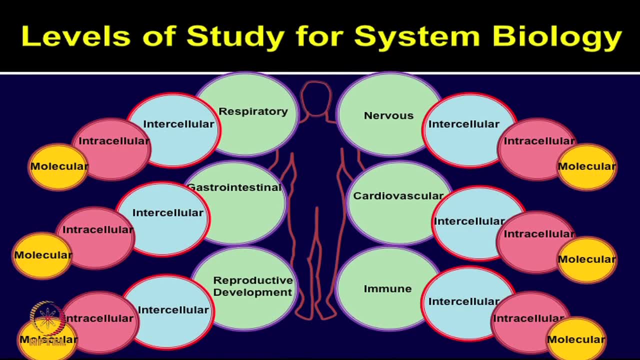 localized in the intracellular dynamics and metabolic networks. These are the vital entities of studying system biology. Now, system biology study can be done at different levels. For example, to study the complex physiology of human, one could look at individual systems such as respiratory nervous system or other physiological systems. Studies can be done. 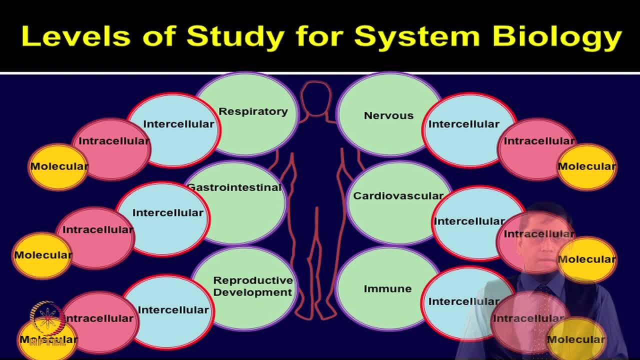 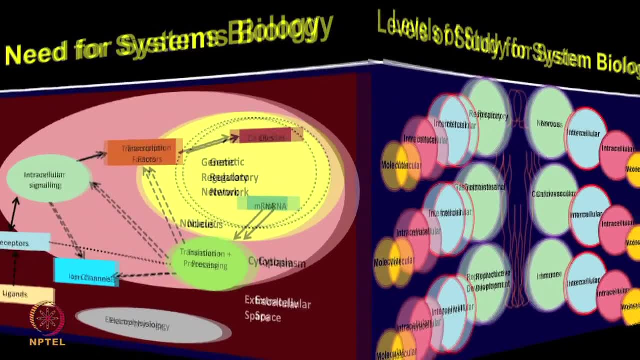 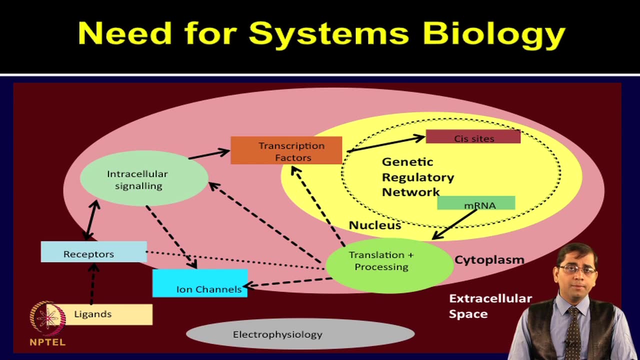 at the intracellular or intercellular level and finally at the molecular level, involving genomics, transcriptomics and proteomics. So why there is need for system biology, The study of biology, The study of biology at the system or subsystem level for understanding the biological processes. 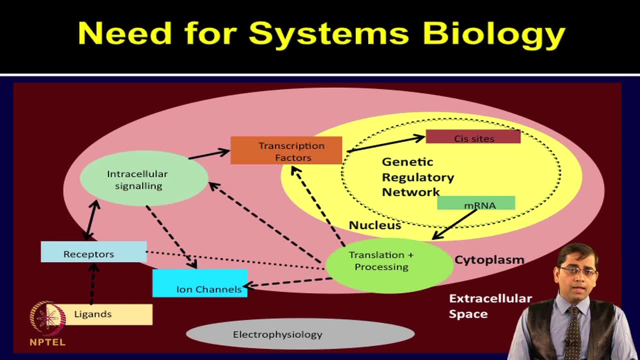 and network is very much required, As you can see in this slide, to understand even simpler system of a cell, how it is regulated with the extracellular space and the cytoplasm and different other components. examination of structure and dynamics of cellular and. 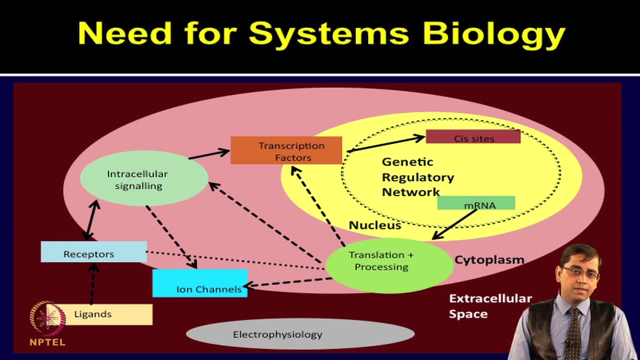 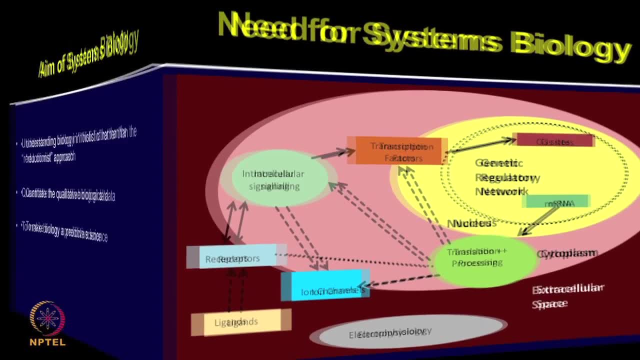 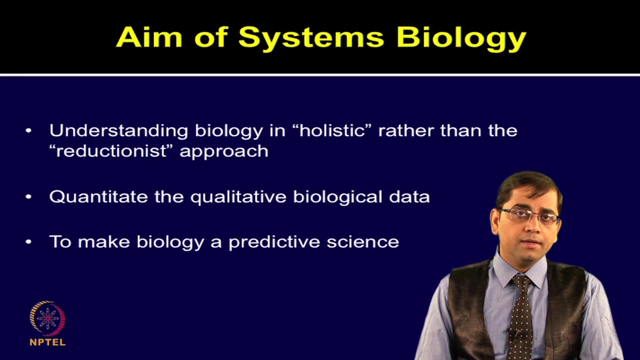 organism function is very much required For understanding of systems rather than characteristics of isolated parts of the cell or the organism. So what is the aim of system biology? To understand the biology in holistic approach rather than the reductionist approach. The system biology aims to quantitate the qualitative biological 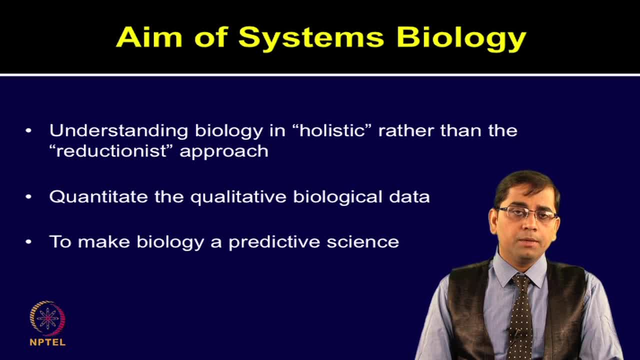 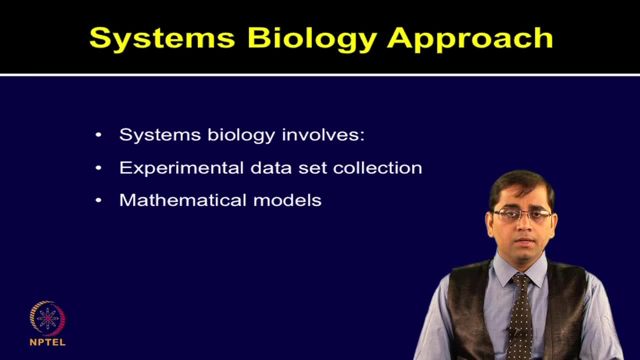 data and provide some level of prediction by applying different types of computational methods. The system biology approach involves, first of all, collection of large experimental datasets and then mathematical models to provide insight of some significant aspects of dataset. The simple system biology approach would involve experiments by adding new datasets which 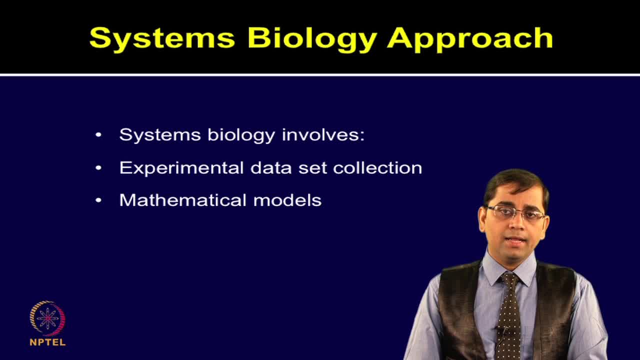 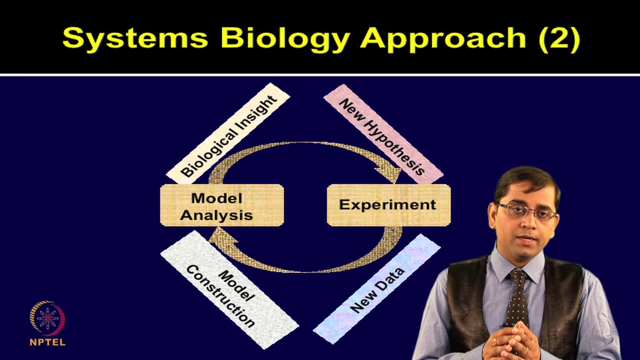 will be used for model constructions and model analysis, And the biological insight derived from these models could be used to prepare a scientific model for an experiment. This used to propose new hypothesis. The properties of systems are probably more than just the sum of all of its individual components. Therefore, it is possible that system may have its own. 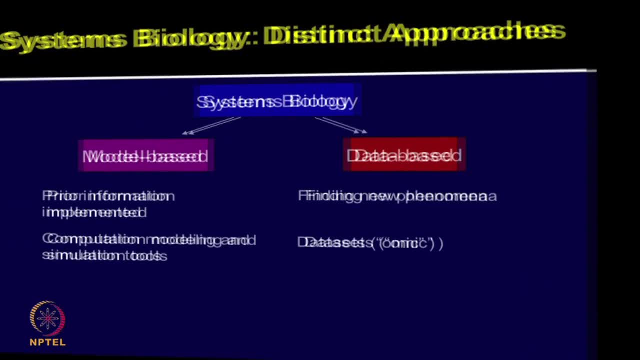 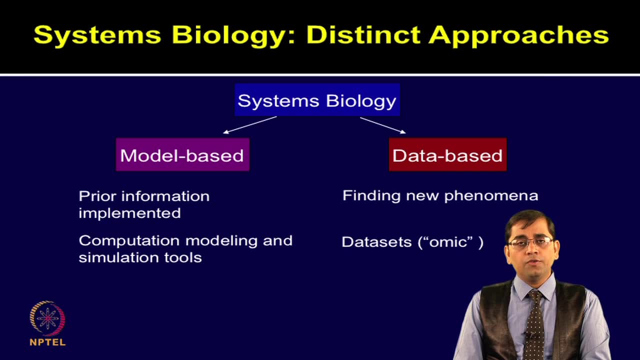 property by applying all the components. So what are the different approaches which have been taken to study systems biology? The different approaches of systems biology include the model based and data based methods. The model based approach involves some prior information which can be implemented in the models, whereas the data based, the objective is to find a 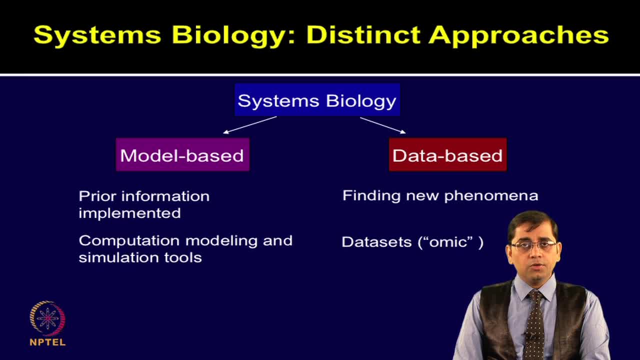 new phenomenon. The model based relies on computational modeling and simulation tools, whereas the data based methods rely on the omics data sets. In model based systems biology approach- it is difficult to build detailed kinetic models, but in data based system the complex relationship among various type of omics, information, metabolic pathways and 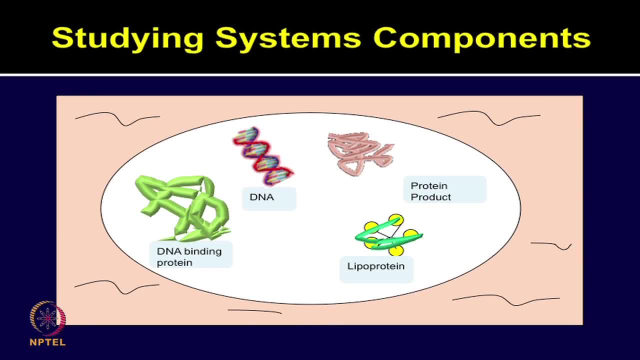 networks can be created. Studying system biology is very challenging. systems biology and biological networks modeling aim to understand the systems structure and function, for better understanding the system's of system properties, like its robustness, as well as its use for prediction of system behavior in response to the perturbations. The reductionist approach involves disintegrating the system. 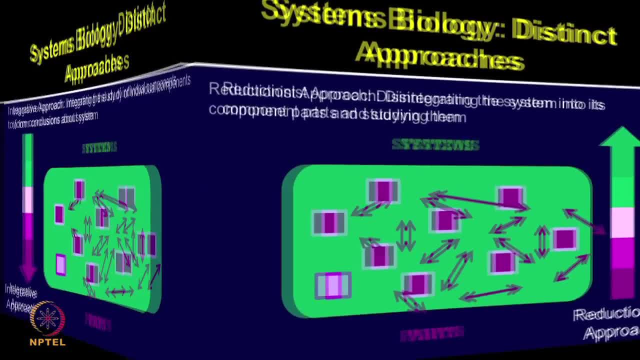 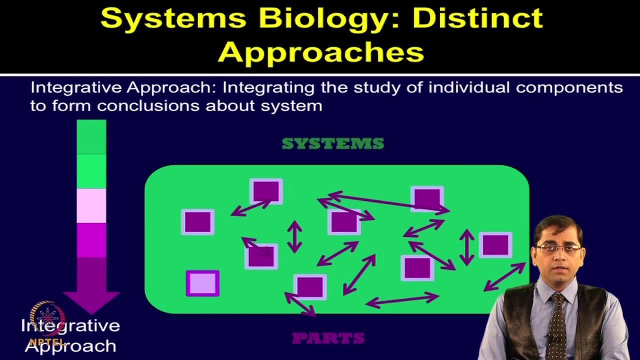 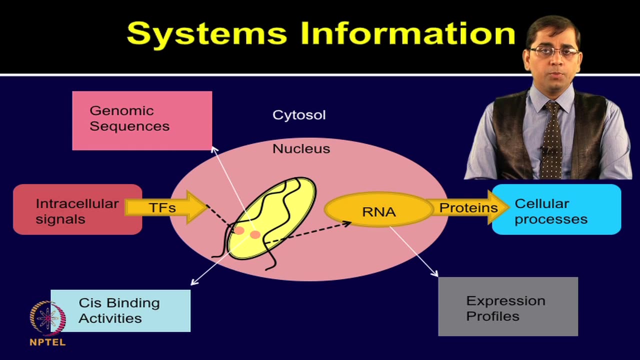 into its component and studying them, whereas the integrative approach involves integrating the study of individual components to form conclusions about the system. Even simpler systems such as cell can be linked with various properties: its genome sequences of different molecules, intracellular signals, transcription factors, different type of cis binding activities. 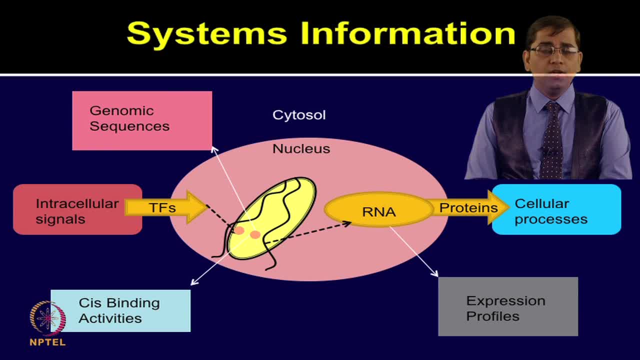 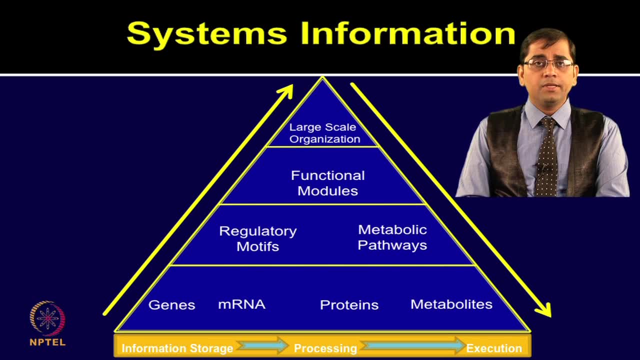 the expression profiling of RNA and proteins and different type of cellular processes. What is system biology triangle? First of all, the systems. information is generated at various level, As we have discussed, starting from genes to mRNA, to proteins, to metabolites, or even identifying regulatory motifs, metabolic pathways, functional modules and different 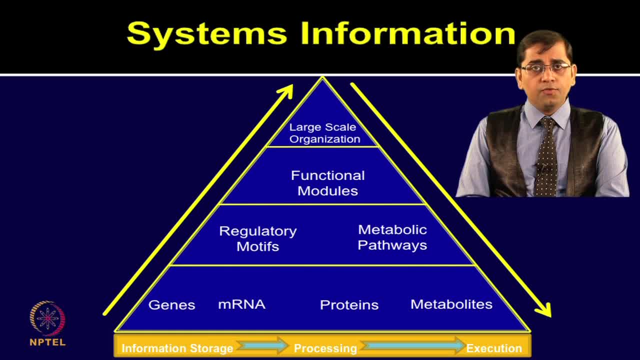 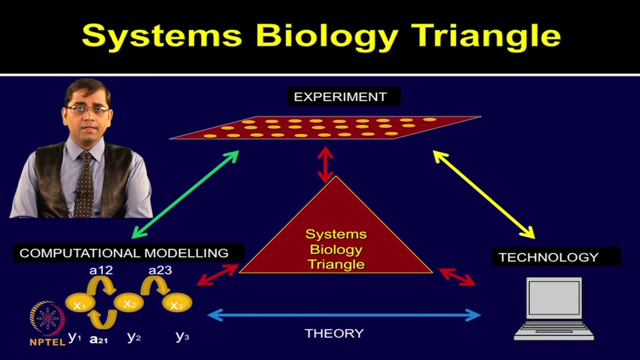 large-scale organizations. This information has to be stored and processed and further executed to identify the system level information energy triangle, as can be seen here, involves the experimental data sets which could be derived from different types of omic technologies How the computational analysis can be. 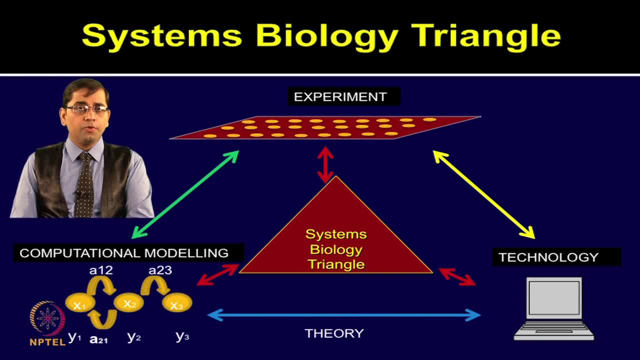 performed different type of bioinformatics software and tools, and then computational modeling by obtaining some theoretical knowledge. The synergistic application of the experiment theory and technology with modeling to enhance the understanding of biological processes as whole system rather than the isolated components, is termed as systems biology. 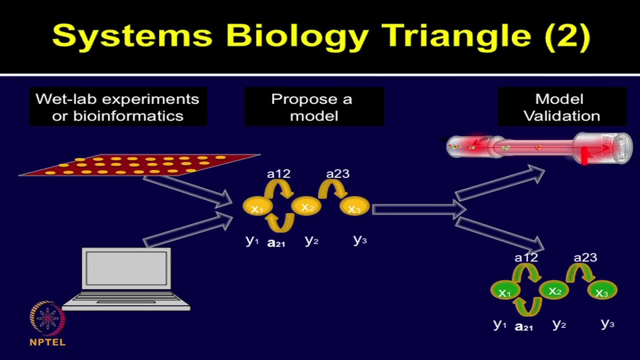 triangle, A systems biology triangle, the wet lab experiments or bioinformatics based data analysis could be used to propose a model, The model building as an aid to understand complex system and some hypothesis could be generated which could be used further to propose more quantitative models or predictive models, and also it can be used for independent techniques for model. 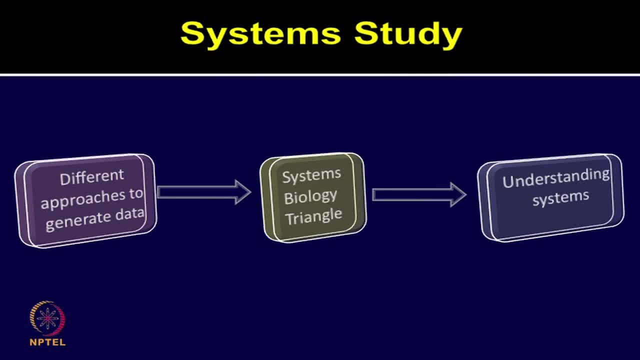 validation. What is system study? First of all, the difference between system study and component should be understood, as discussed earlier. After generating the data set and creating the systems biology triangle, This information could be used for understanding the systems in more complex and mechanistic. 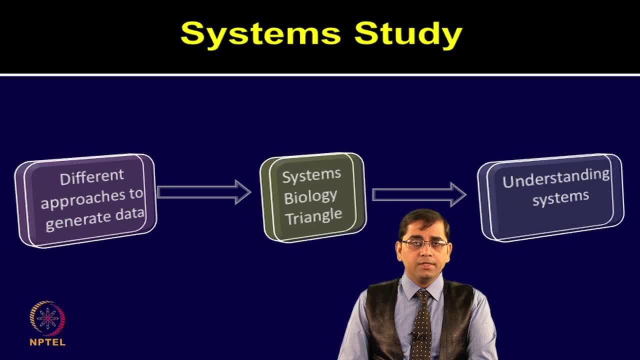 level. So what approach one could take to study about the systems extracting and mining the complex and quantitative biological data, integration and analysis of these data sets for development of mechanistic, mathematical and computational models and validation of these models by retesting, retesting and refining, after proposing some hypothesis, Different online databases and 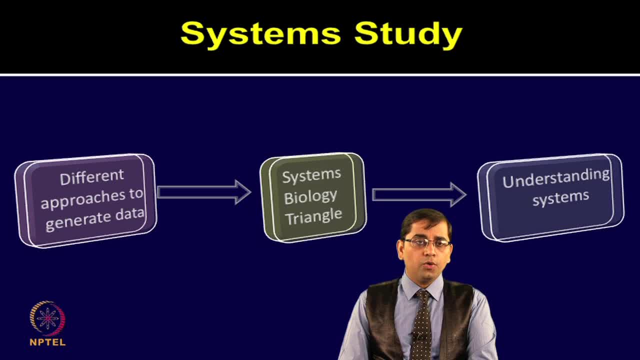 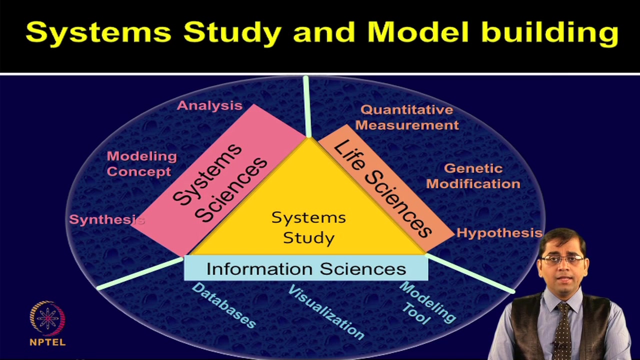 repositories are nowadays developed and available for sharing large data sets and various systems model. The systematic approach how molecules act together within the network of interaction that make up life is definitely going to be useful to understand the systems. biology, System study and model building. the system science includes synthesis. 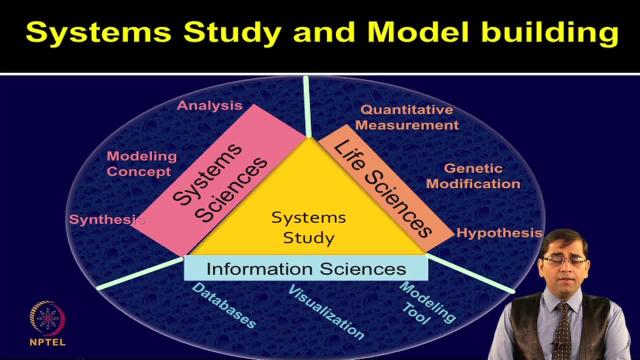 modeling, concepts, analysis. Life science disciplines provide quantitative measurements, genetic modifications and deriving some hypothesis. The information science enables the visualization, the modeling tools and different databases. This model building as an aid to understand the complex system is very useful for system level investigation. There are different technologies. 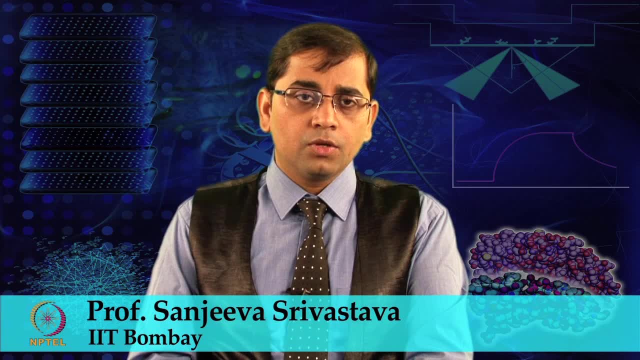 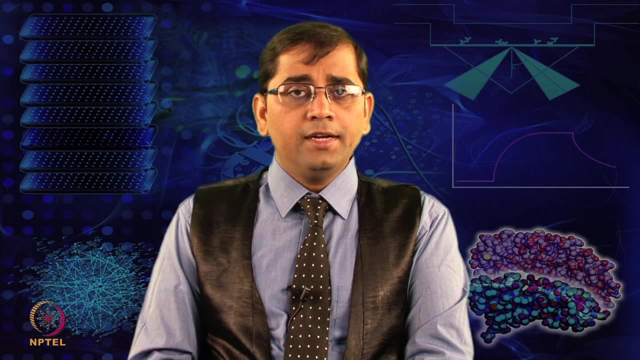 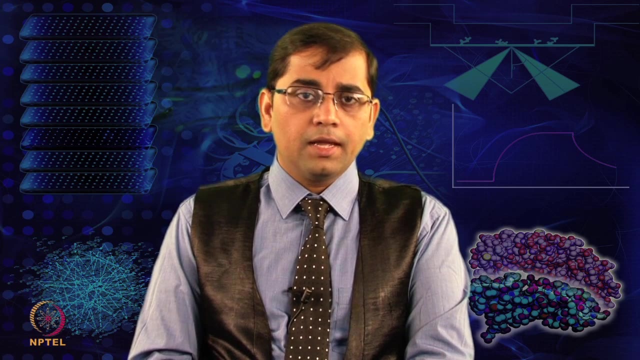 which have been employed to study the systems biology. Obviously, we need high throughput data set, which could be derived from microarray platform or RNA, deep sequencing, different configurations of mass spectrometry, different type of proteomic tools and protein interaction data sets. Some of the technologies which are commonly 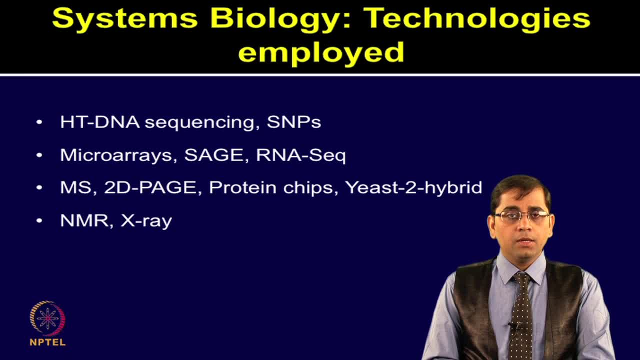 employed in system biology could be classified broadly under the following techniques For genomics: there are high throughput DNA sequencing methodologies. mutation detection using SNP method For transcriptomics. the transcript measurements can include serial analysis of gene expression, gene chips, microarrays and RNA sequencing. 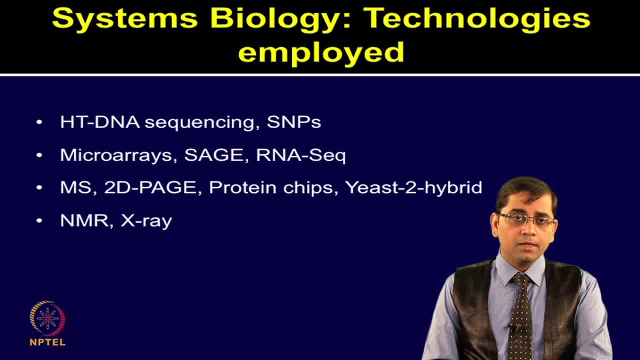 For proteomics: mass spectrometry, two dimensional electrophoresis, protein chips and yeast, two hybrids, and different structural proteomic tools such as X-ray and nuclear magnetic resonance, X-ray and NMR are mainly employed for metabolomic analysis. in the field of metabolomics, 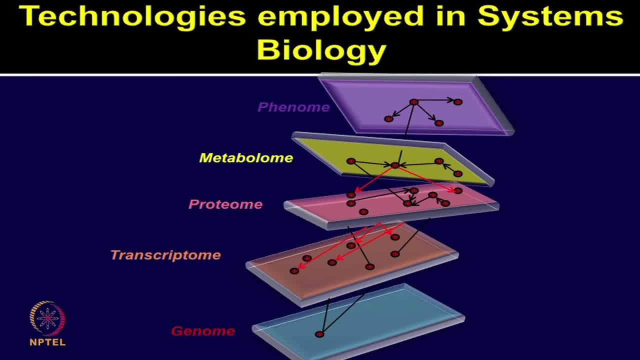 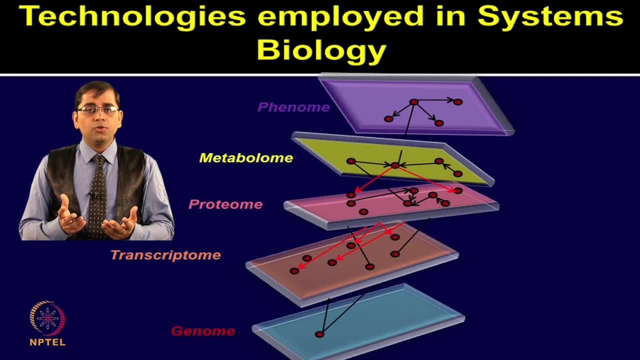 For some types of information. the systems study requires different technologies which could be employed at different levels in biological systems, At genome level, by studying different type of technologies such as high throughput sequencing, high throughput arrays, transcriptomics, transcript analysis using RNA sequencing and microarrays, Proteome- we have discussed 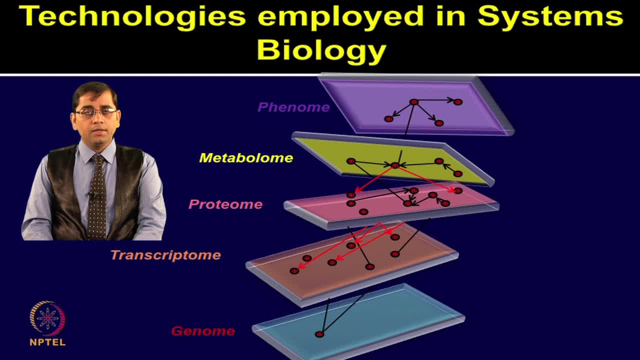 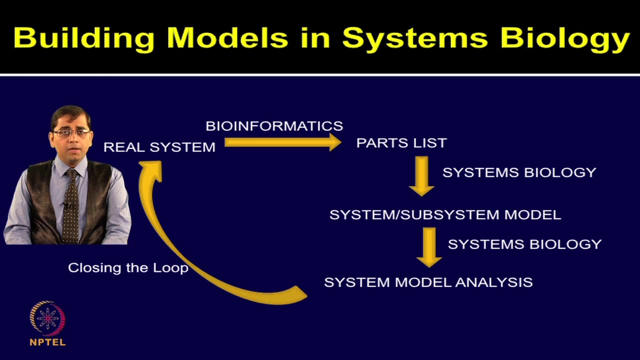 methodologies: Metabolome could be performed using either NMR or mass spec and in phenome, studying the images by using NMR method. Each level of these omic technologies could be useful for studying systems biology. Let us now talk about how to model biological networks, To build a model in systems biology. 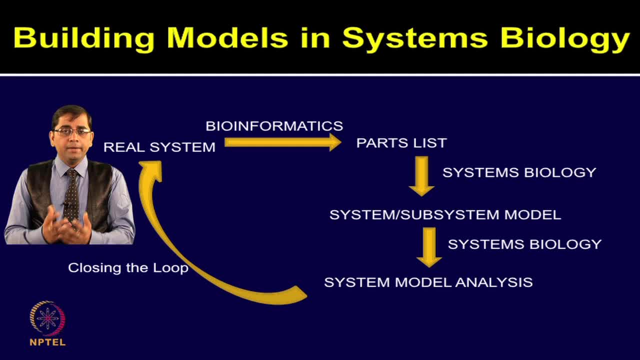 first of all, all parts can be generated. by the data sets derived from systems biology approach, The system or subsystem model can be generated which could be used for systems model analysis. Now this could be applied for real systems and by applying knowledge using bioinformatics tool, it could be applied again back to the original components, which 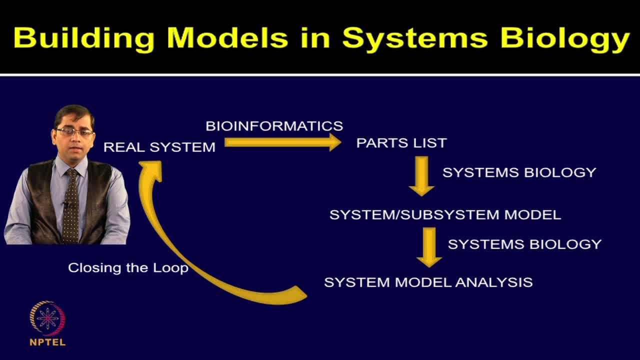 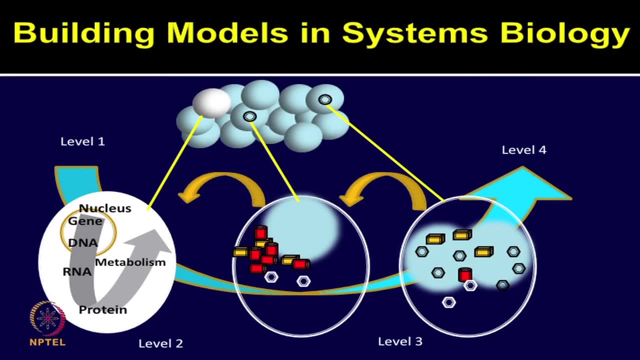 can be used to derive some hypothesis, and validation of these data sets could be performed. It will work like a closed loop To build the models in systems. biology information is generated at different level. Level one, such as DNA and gene expression. level two, the intracellular. 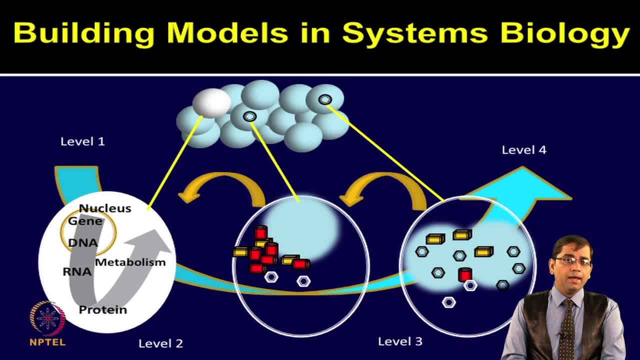 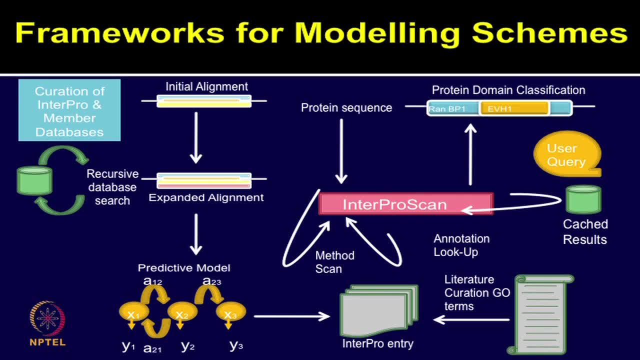 networks. level three, cell, cell and transmembrane signals. and level four, integrated organ level information. What are the frameworks required for modeling schemes? Different types of deterministic or stochastic models have been proposed. The compartmental variables or individuals or functional variables have been studied, Especially homogenous or especially explicit. 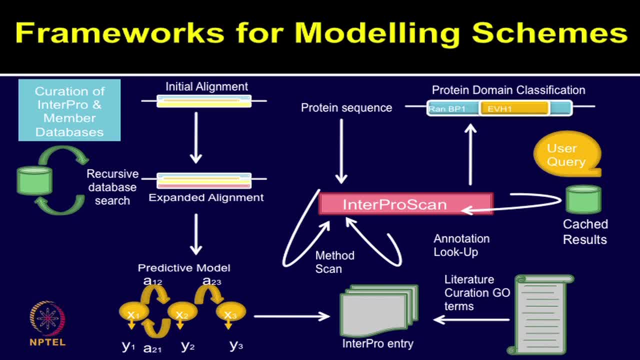 models are generated which could be applied in the uniform time scale or separate time scale. This framework could involve single scale entities or cross scale entities. As you can see in the slide, this framework requires different level of information in very complex manner, Whether it is curation of the data bases, how to align these information using 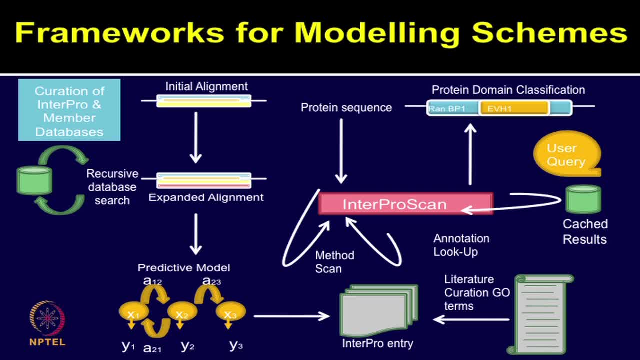 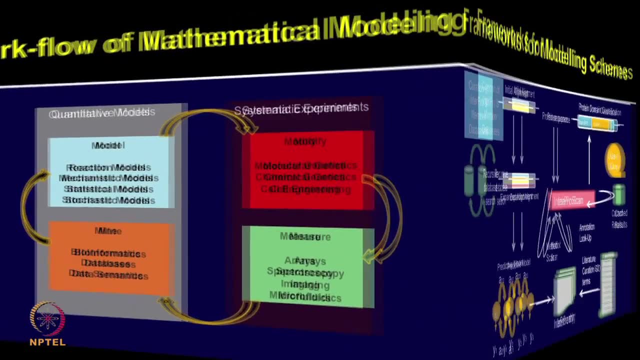 bioinformatic tools to generate the predictive models, which could be also developed by using the literature, curated data sets or experimental data sets. and, finally, it could be used to study the system level properties. Let us discuss the work flow of mathematical modeling. A paradigm can be proposed based 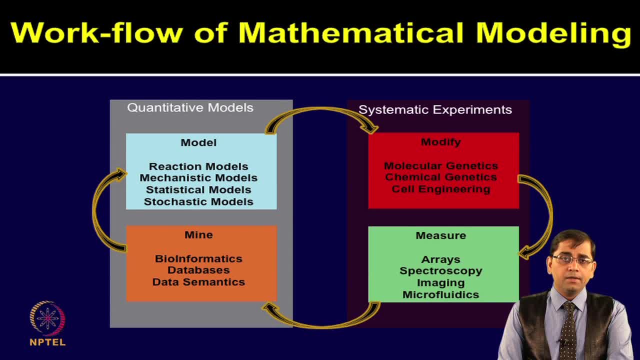 on: modify, model, measure, mine, Systematic experiments, different type of molecular genetics, chemical genetics and cell engineering approaches could be used to modify and different level of measurements by applying microarrays, spectroscopy, imaging, microfluidics based approaches from proteomics and genomics which could be used further for mining, which involves bioinformatic. 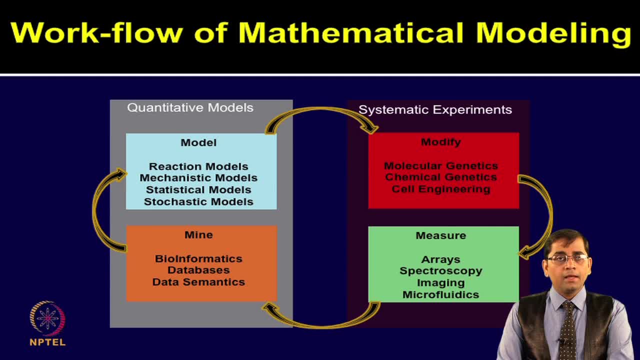 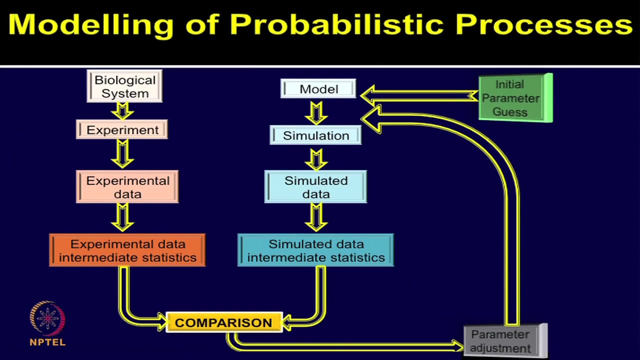 data bases and data semantics. Now these sets could be used to derive the model, which could be reaction, mechanistic, statistical or stochastic models. Starting from systematic experiments to reaching and deriving the quantitative models, this work flow can be applied. The modeling of probabilistic processes involves 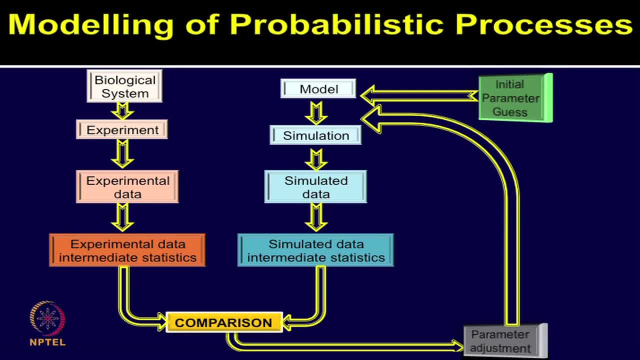 let us say you want to study a biological system, So some experiment has to be performed. the experimental data set will be generated, from which some statistics could be applied which can be used for comparison. Now, different type of models can be generated using simulations. 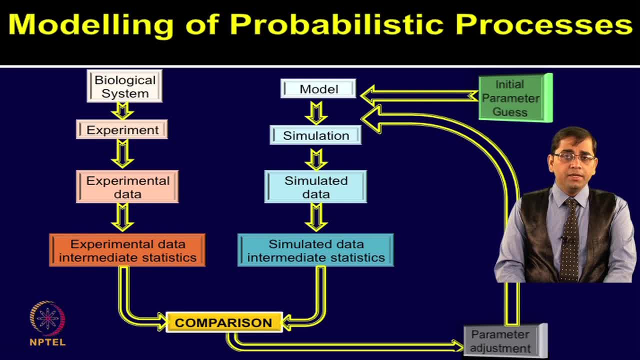 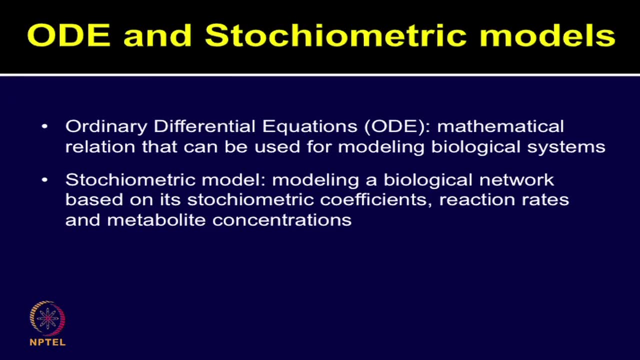 and simulation data sets which can be used for intermediate statistics. by comparing these two types of information and adjusting the parameters, one can study the systems and derive probabilistic processes. What are ordinary differential equations and stoichiometric models, The quantitative analysis measures and names to make models for precise kinetic 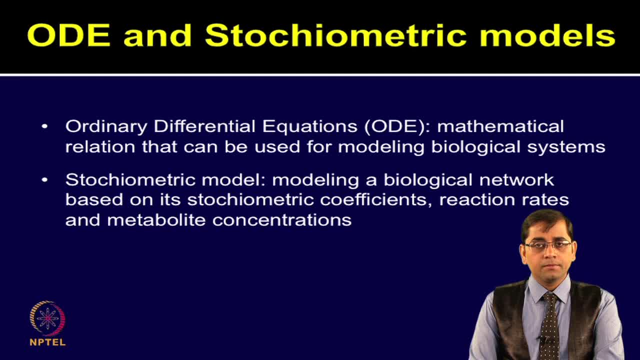 parameters of a systems network component. It also uses properties of network connectivity. ODE is a mathematical relation that can be used for modeling biological systems. The classical models mostly use ODE to link reactants and products concentrations through the reaction rate constant to develop the computationally efficient and reliable models of the underlying. 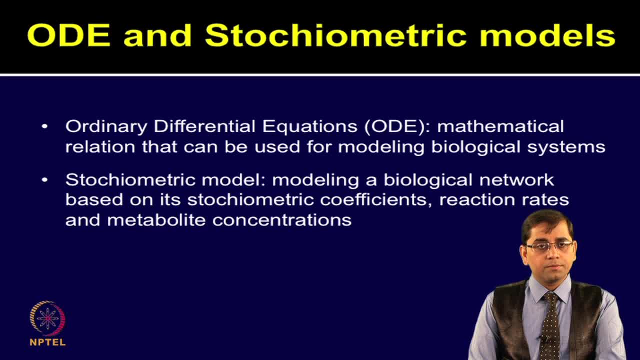 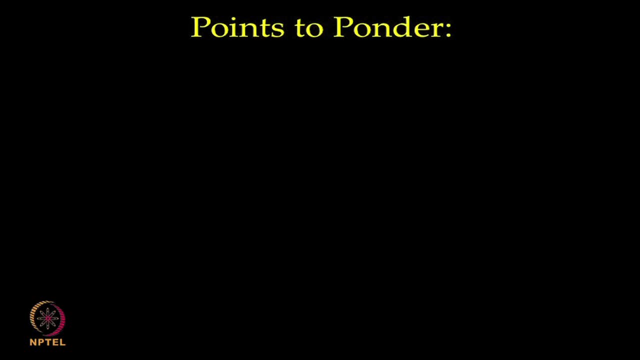 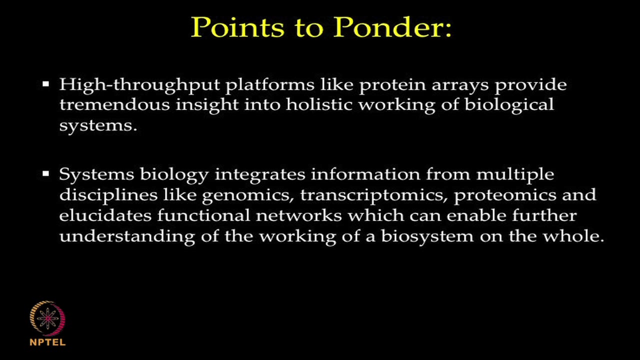 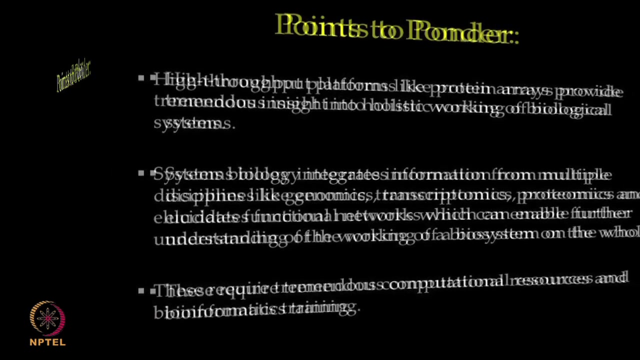 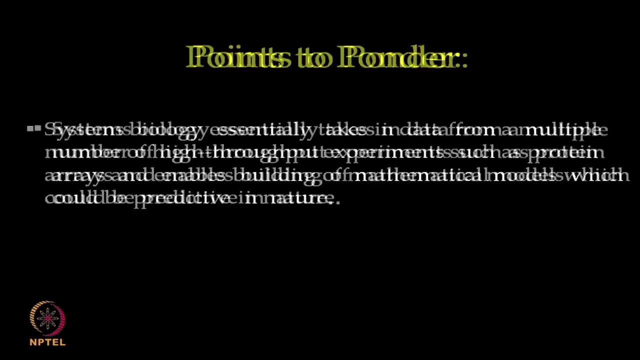 gene regulatory networks. these ODE models could be used. the stoichiometric model: it is a modeling, a biological network based on its stoichiometric coefficients, reaction rates and metabolic concentrations. The micro faculty is Beh ciudad and are, So in this lecture you understood the various challenges associated with the protein array. 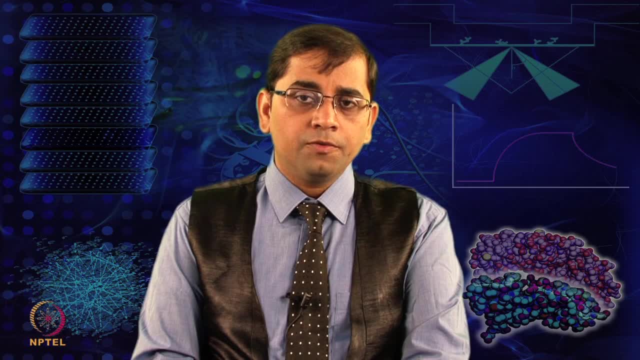 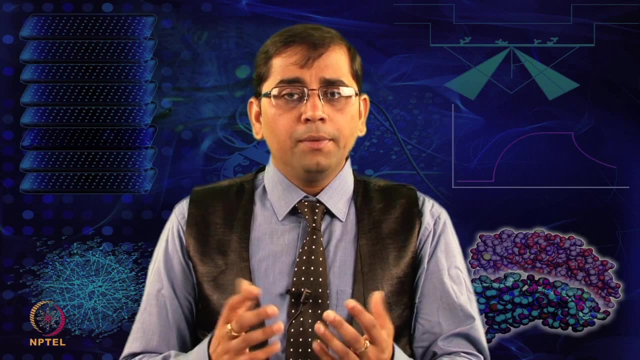 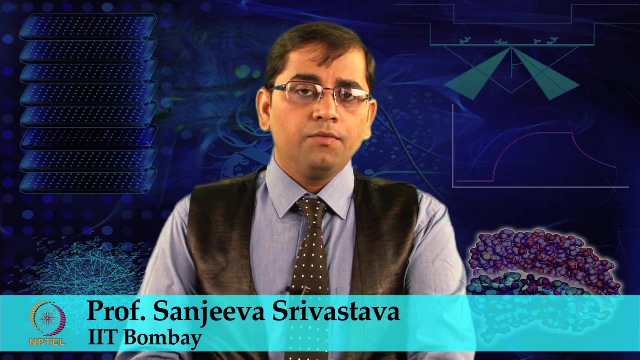 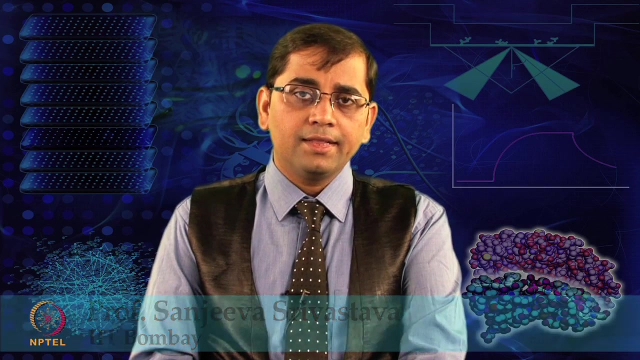 workflow. You were introduced to the basic concept of systems biology, which are helping new age researchers to integrate data from the multi-omics resources and pure sciences to understand biological organism systematically. With these foundation concepts, we will look at some advanced skills of systems biology in the next lecture. Thank you,